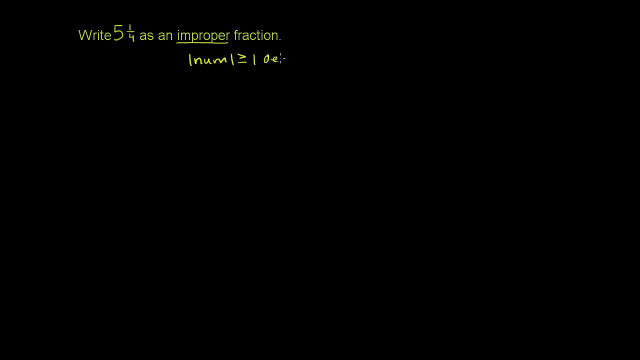 is greater than or equal to the absolute value of the denominator. I could have just shortened it, but you get the idea. The numerator is greater than or equal to the absolute, or the absolute value of the numerator is greater than or equal to the absolute value. 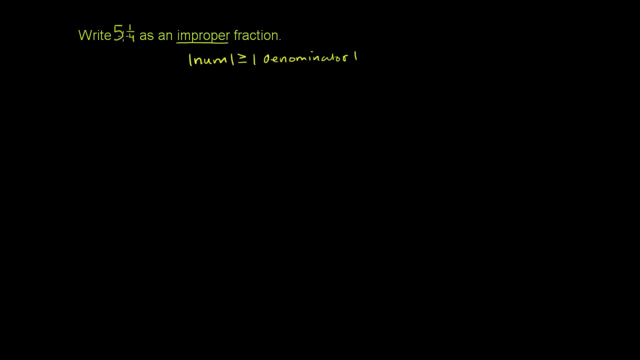 of the denominator. In this situation, right here, it's a mixed number. We have it as a combination of 5, which is just a whole number, and 1, fourth, which is a proper fraction, because the numerator is less than the denominator. 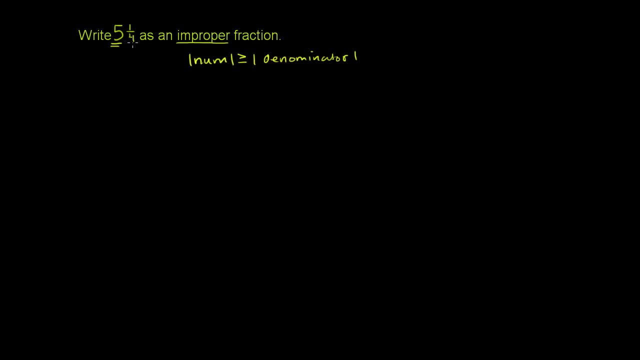 The absolute value of the numerator is less than the absolute value of the denominator. So to write it as an improper fraction and I'll show you kind of the methodology for doing it, and then we'll talk a little bit about why that methodology works. 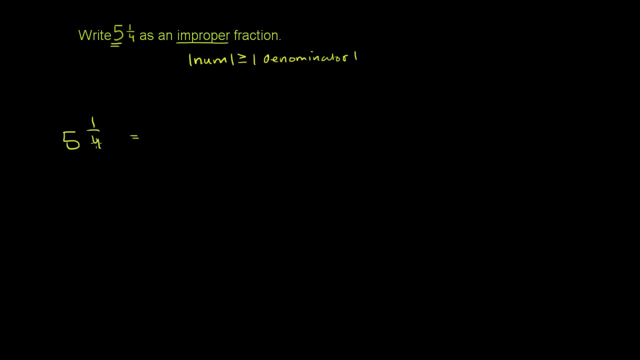 So 5 and 1. fourth, The methodology is pretty straightforward. You say, OK, 5, the whole number 5, that is the same thing as 20 over 4.. And so 20 over 4 plus 1 over 4 is 21 over 4.. 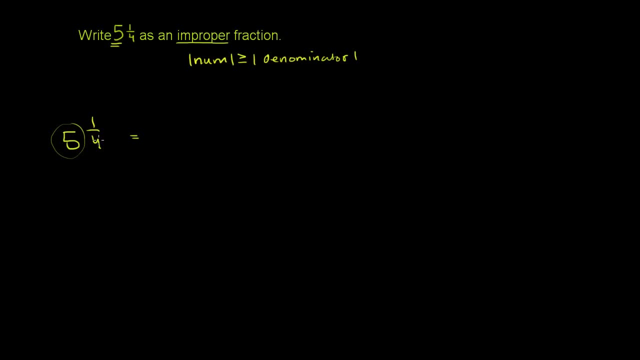 Or another way to think about it is: 5 times 4 is 20, plus 1 is 21,, 21 over 4.. So that's the methodology, Pretty straightforward, And I'm going to draw it out so it makes a little bit more. 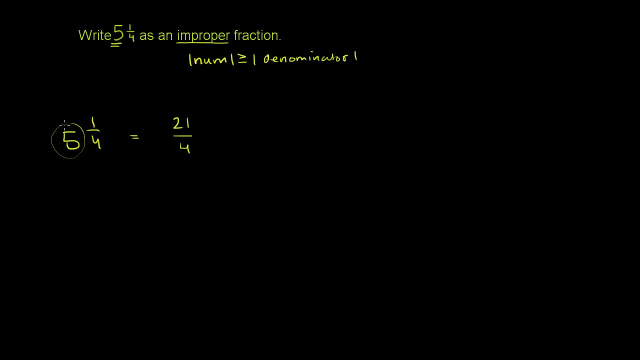 sense. So once again, you take the mixed number, or you take the whole part Of the mixed number. You multiply it times the denominator, you get 20.. And then you add that 20 to 1,, you get 21 over 4.. 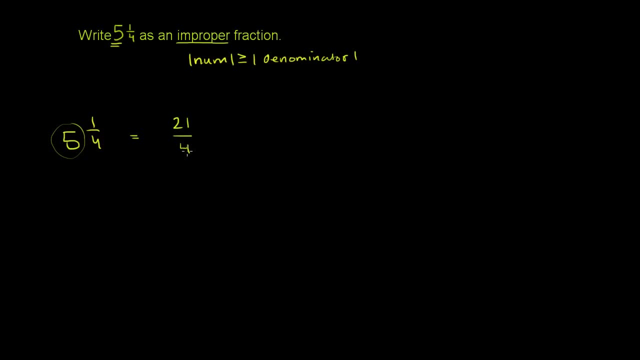 And now it's an improper fraction. The absolute value of our numerator is greater than the absolute value of our denominator. Now I do want to show you why this works. So, to see why this works, let's think about what 5 and 1? 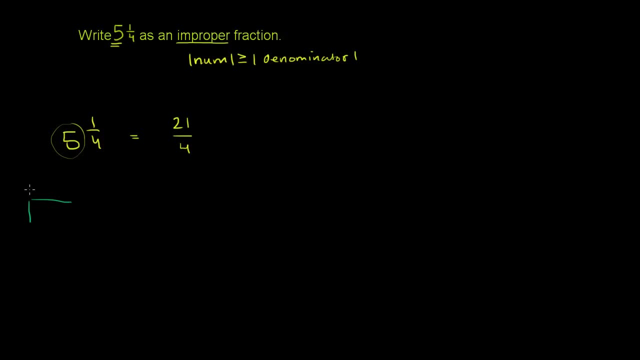 fourths means It means we have 5 wholes. So let's say that this is a whole, So that's one whole, And let me copy and paste it five times. So copy, and then let me paste it, So that's 2,, that's 3,, that's 4, and then that is 5.. 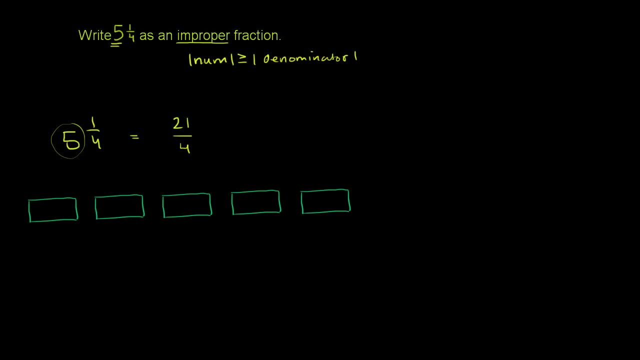 So we have 5 wholes. So that's this stuff that I've drawn in green. That's 5 wholes right there. And then we have 1 fourth, So I'll do 1 fourth of a whole. So 1 fourth of a whole will look like that. 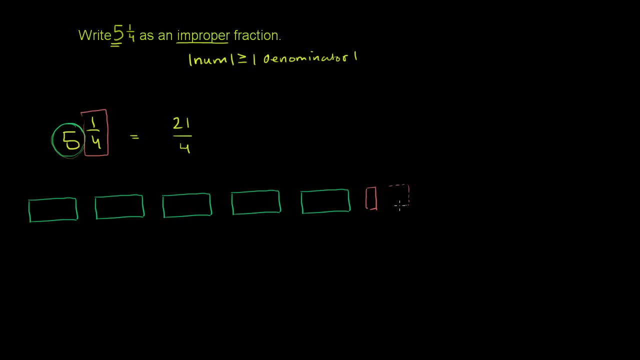 And just to be clear that it's part of a whole. I could have drawn the whole in a dotted line to say that we don't have that whole. We have only 1 fourth of it And that's that 1 fourth. So this is 5 and 1 fourths. 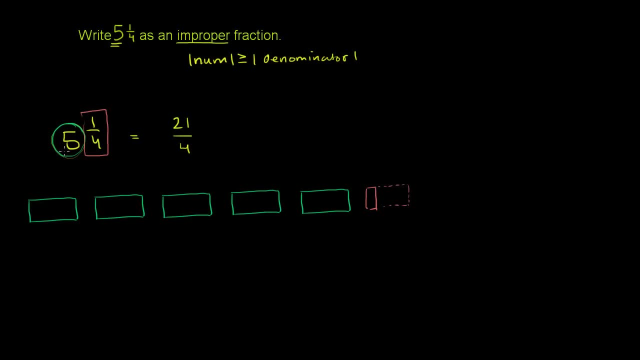 So, to write it as an improper fraction, you can really view this 5 as some fraction over 4.. And, to think of it that way, divide each of these into fourths, Or this is one way to think about it. So this right over here is 4 fourths. 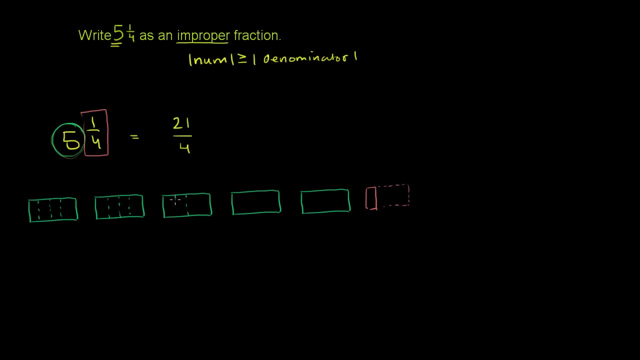 This is another 4 fourths. This is another 4 fourths. I should have copied and pasted this. This is another 4 fourths, And this is another 4 fourths. So now, how many fourths do we have? 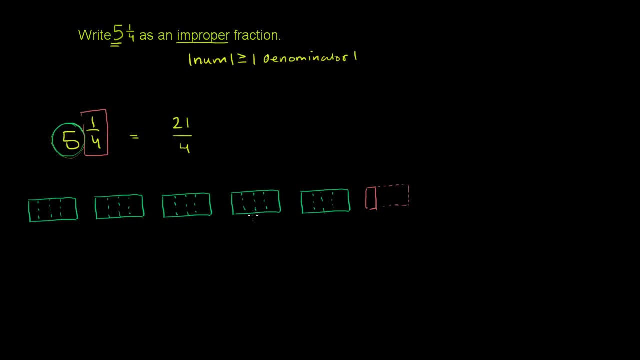 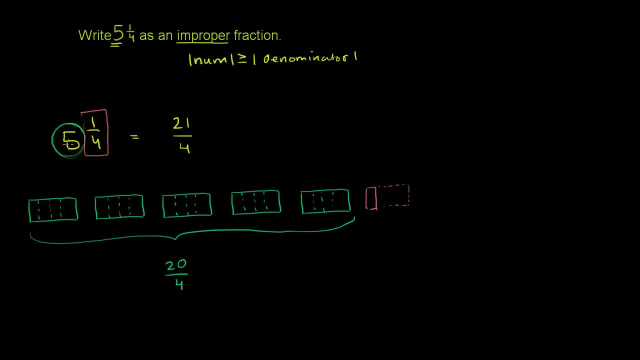 That's what we have in green right over here. That is the same thing as 5.. Each of these are 4 fourths, So you could view this as 5 times 4 fourths. 4 fourths is 1.. 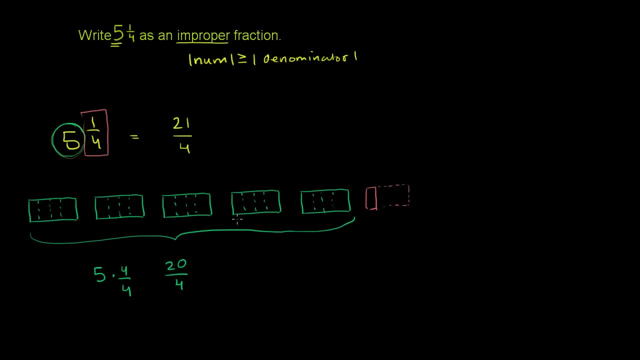 5 times 4 fourths is 20 over 4.. That's what we have right over here. And then now we can add it to that 1 fourth. Now you can add it to that 1 fourth and you will get 21.. 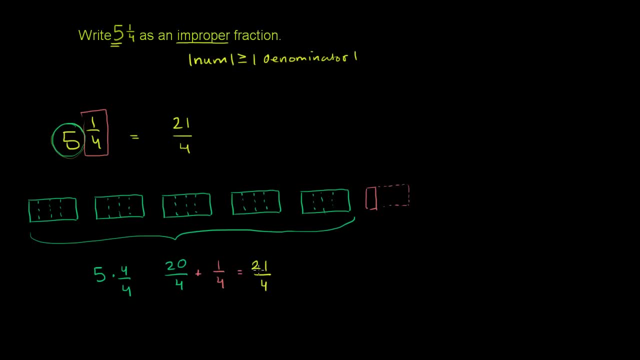 We have the same denominator so we can just add the numerators 21 over 4.. So that's the conceptual Understanding of why it works. but when you see any mixed number it's a pretty straightforward process. Multiply the 5 times 4.. 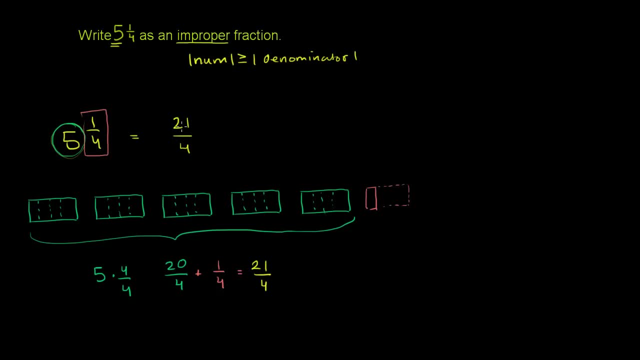 You get 20.. 20 plus 1 is equal to 21 over 4.. And actually let me just write that out just so you get clear on what I'm doing. So 5 and 1 fourths, that is the same thing. 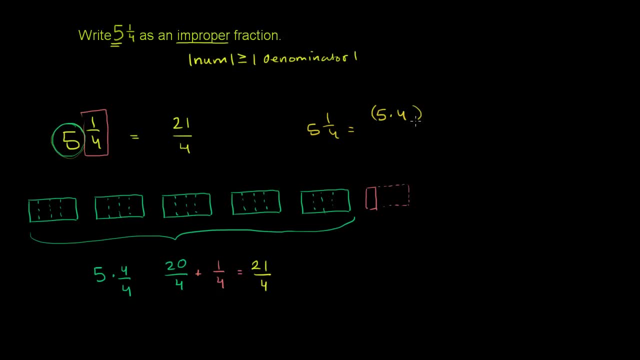 as that's equal to 5 times 4 plus 1 over 4.. And this is why.